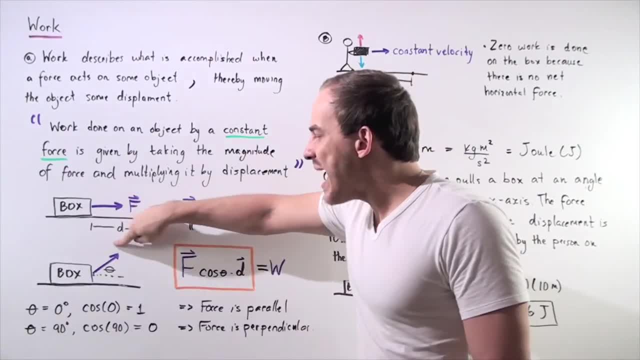 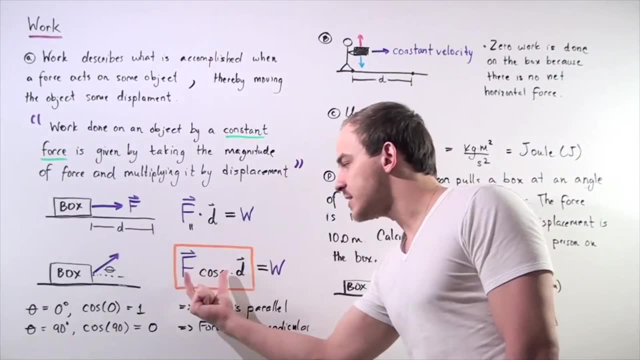 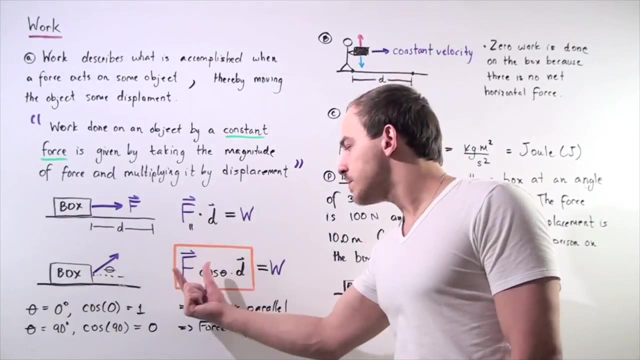 acted prior. So now we simply take the magnitude of this force, f, and multiply by the cosine angle, theta, and this gives us the x-component of the force that acts in the same direction as displacement. So I multiply displacement by my x-component force and I get my work. 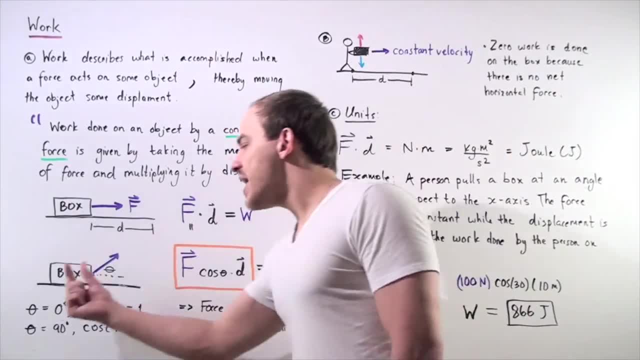 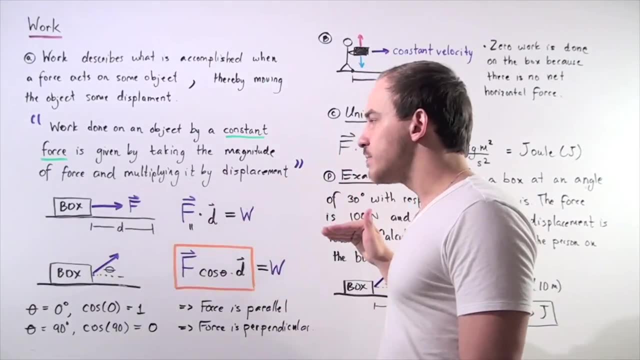 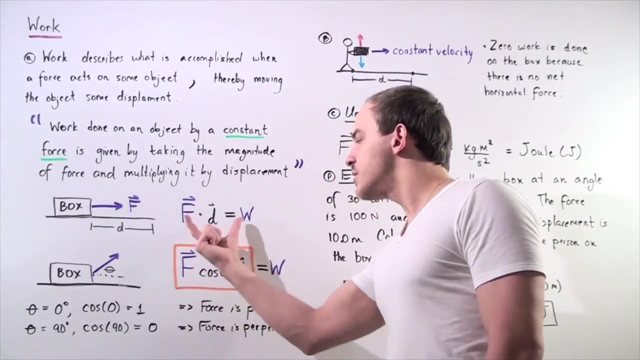 done So once again. when the angle is zero degrees, what happens is The force acts in the same direction as displacement, and because cosine zero is one, this cosine of zero simply becomes this formula. So this formula simplifies to this formula when the 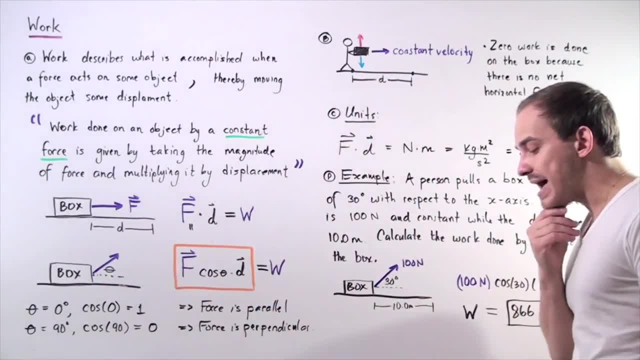 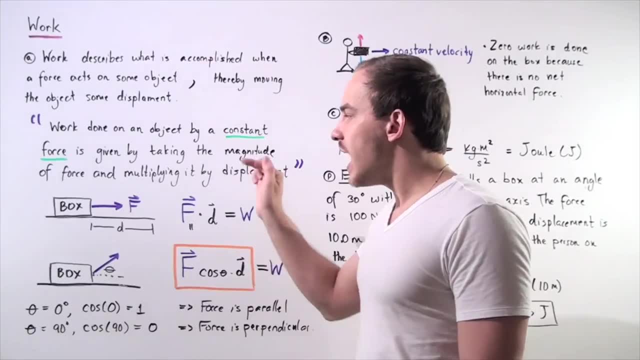 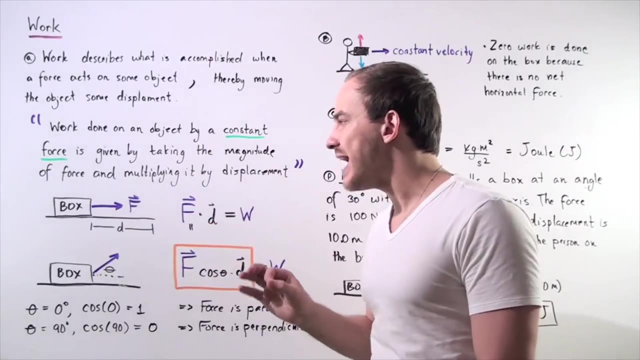 cosine of the angle is zero. So that makes sense mathematically. What about when the cosine is 90?? So that means the angle acting on the object or the force acting on the object is 90. Now we know that the x-axis is perpendicular to the motion, to our displacement and in 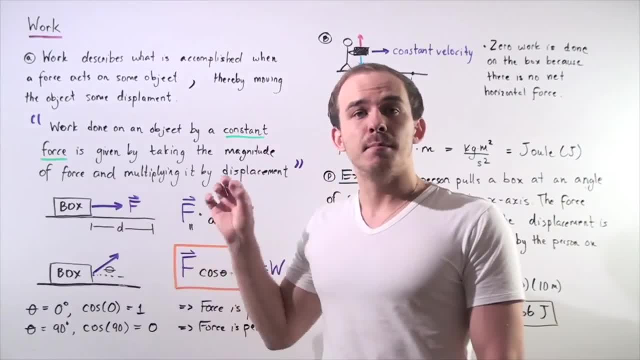 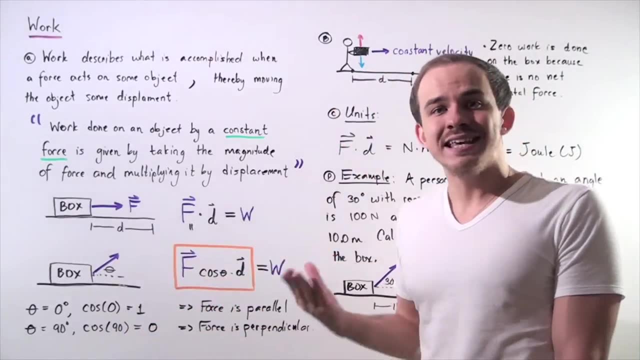 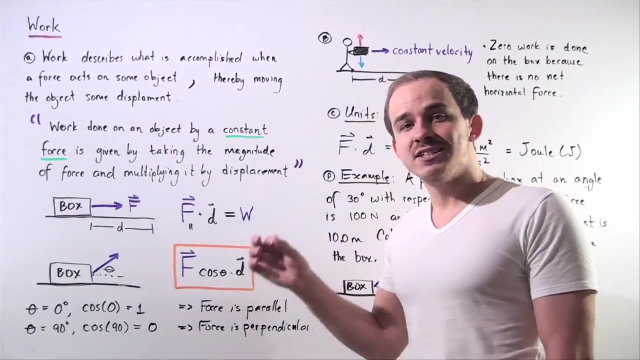 this case, no connection or no work is done on the box. And this makes sense mathematically because cosine of the angle 90 is zero, So this whole term becomes zero, and so whenever we have a force acting at a 90 degree angle to our displacement, zero work is done. 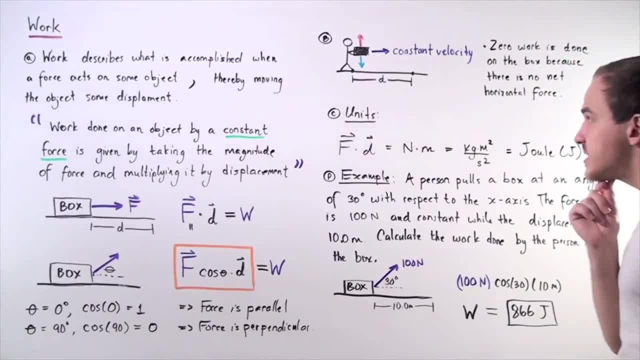 So let's look at the following example. Let's suppose that we were going to get the force acting on the object. So what would happen if the force acting on the object was 90 degrees? let's suppose we have a person, the person is carrying a box and that person is moving with 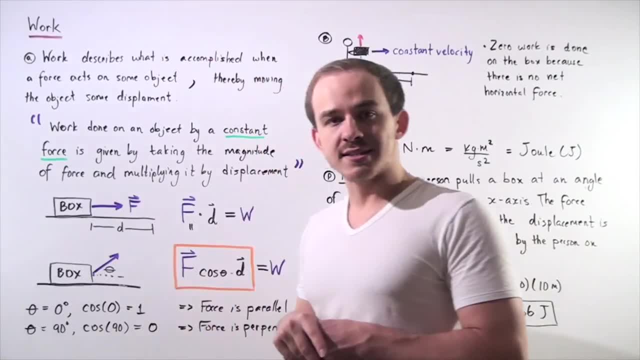 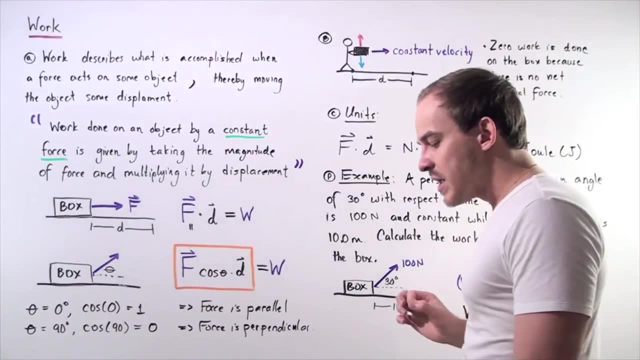 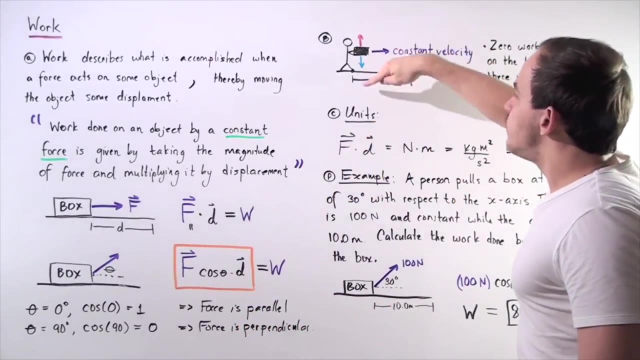 constant velocity along the x-axis. So that means because we have constant velocity, the box is moving with constant velocity and that means we have a net force of zero. So notice that the only forces acting on the box are forces pointing along the y-axis. We have the force of gravity. 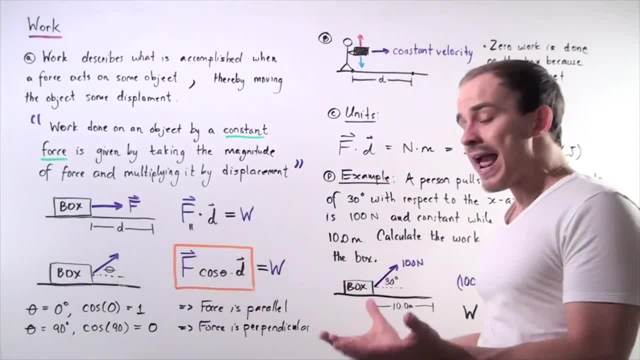 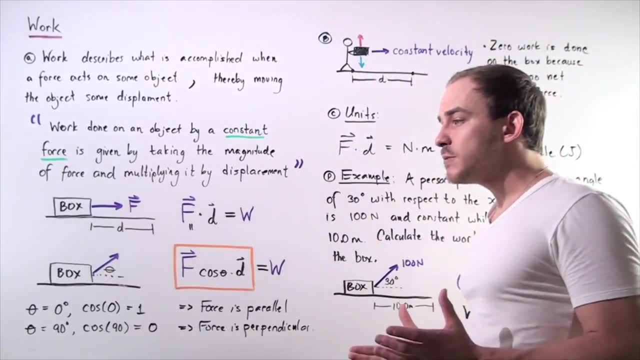 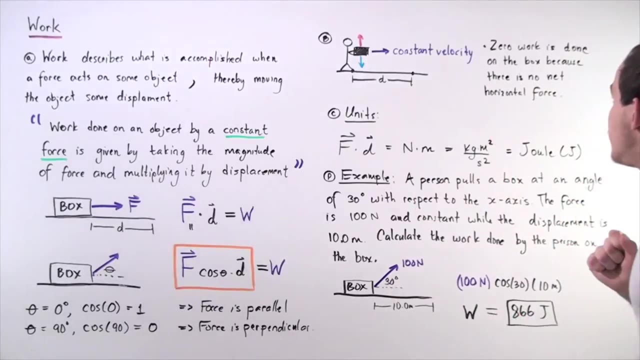 pulling downward on the box and the force our hands create on the box that point in the opposite direction of motion. So we have no displacement along the y-axis, so no work is done along the y-axis. And likewise, because we have a net force of zero, zero work is done along the x-axis. 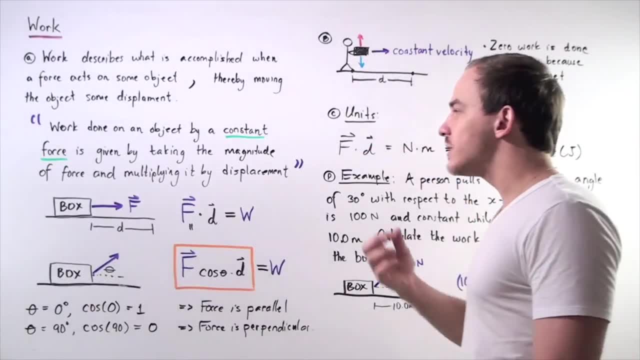 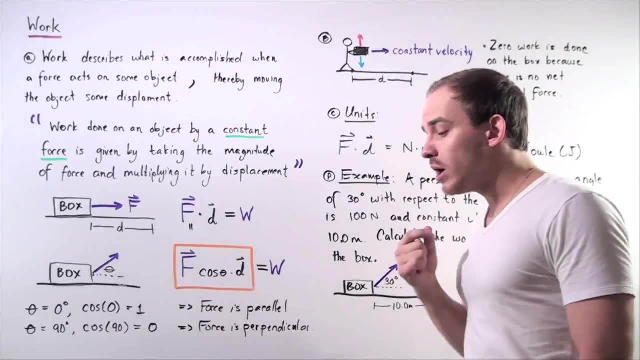 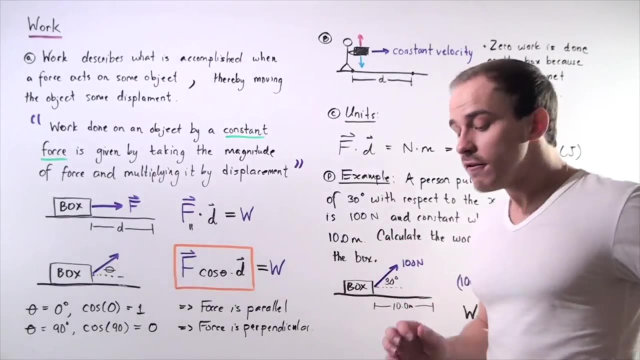 So, even though we have displacement, no work is done along the x-axis because our net force is zero. Now, if we want to actually pick the box up from the ground, work is done at that moment because the force we're applying, the net force we're applying on the box, acts in the same. 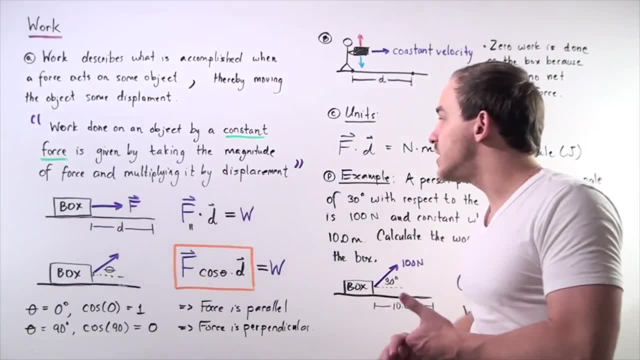 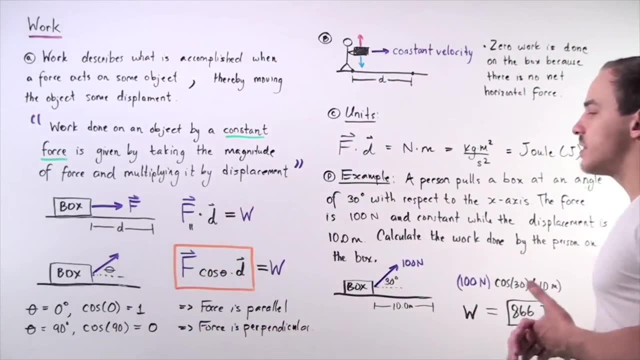 direction as displacement, and so work is actually done. But when we're holding the box still and walking with the box, we're not doing any work. So we're not doing any work, So we're not doing any work. So when we're holding the box with constant velocity, no work is done on the box. So 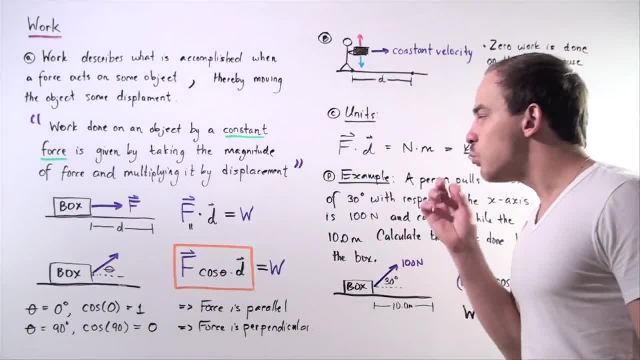 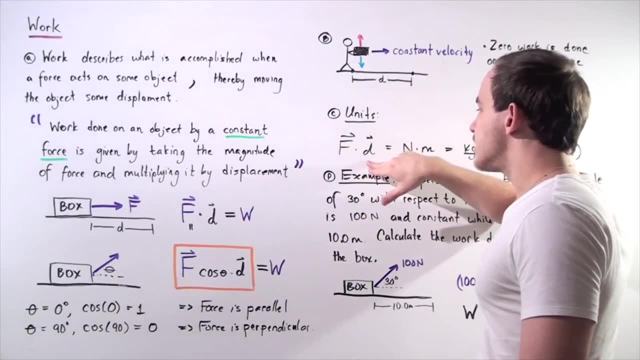 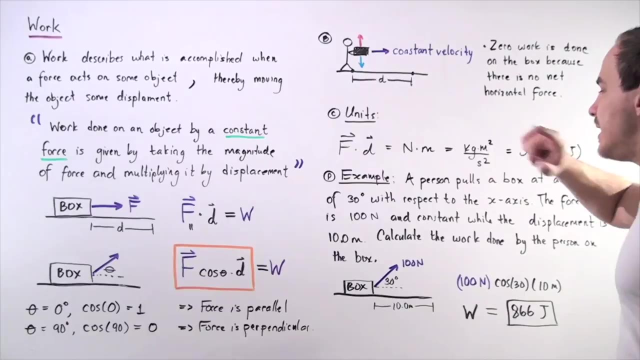 we said earlier that work is a scalar. But what are the units of work? Well, work is given by taking the force and multiplying by distance. And since force has newtons and displacement is given in meters, then our work is given in newtons times meters, which is the same thing. 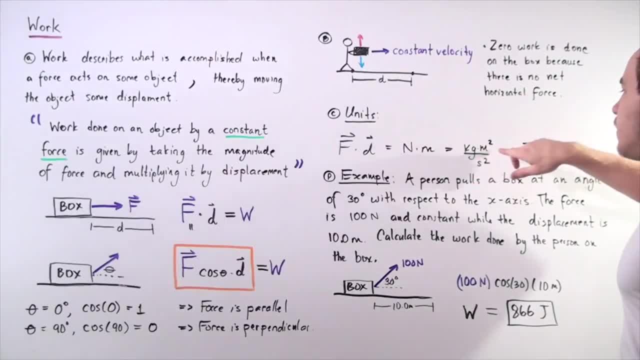 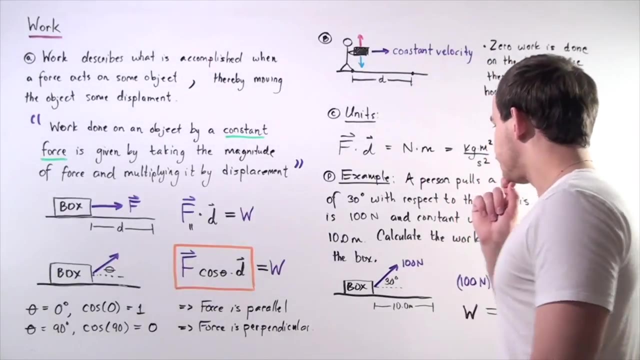 as saying kilograms times meters squared divided by seconds, And this unit is known as joule, given by the following J symbol. So let's look at the following example and let's calculate the work done on a box. A person pulls a box at 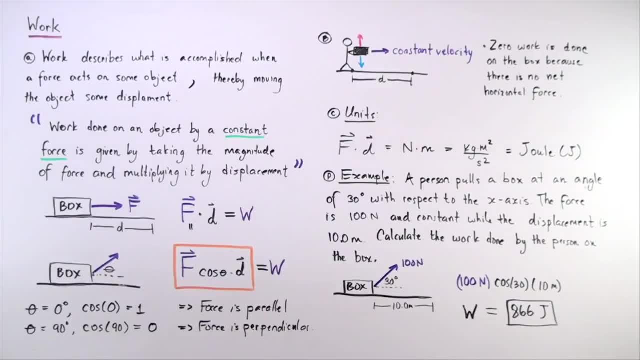 an angle of 30 degrees with respect to the x-axis. with respect to the motion of the box, The force is 100 newtons and constant, while displacement is 10 meters. Calculate the work done by the person on the box, So here we have the diagram. So our box is displaced. 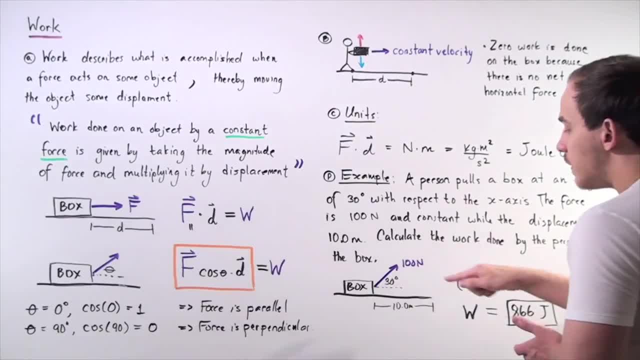 a displacement of 10 meters and the force of 10 newtons is acting at an angle of 30 degrees with respect to the motion, with respect to our displacement. So that means we have to find the x-component of the force, because we must find the force that's acting parallel. 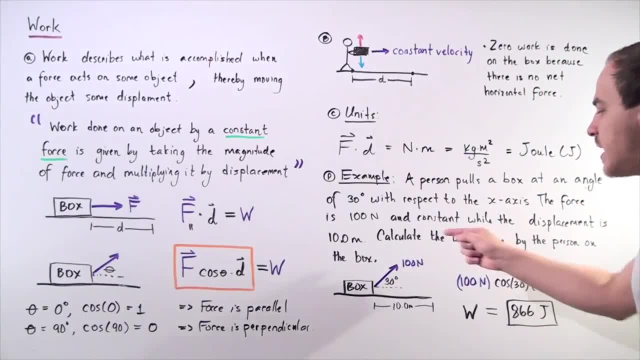 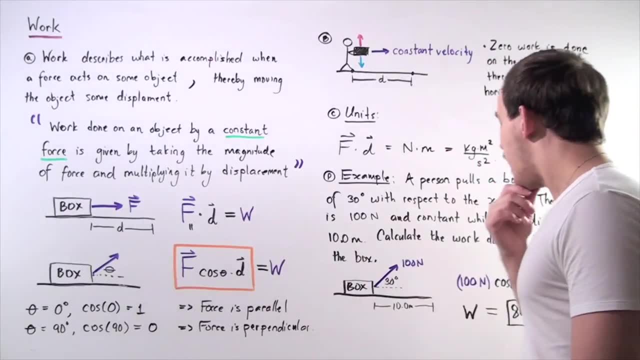 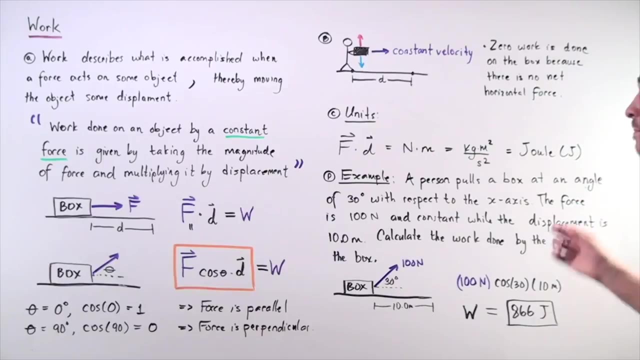 to the displacement of the object. So we take cosine of the angle 30, we multiply it by 100 newtons and we multiply it by our displacement of the box and we get approximately 866 joules of work is done by the person on the box to move the box, displace the box a distance. of 10 meters.